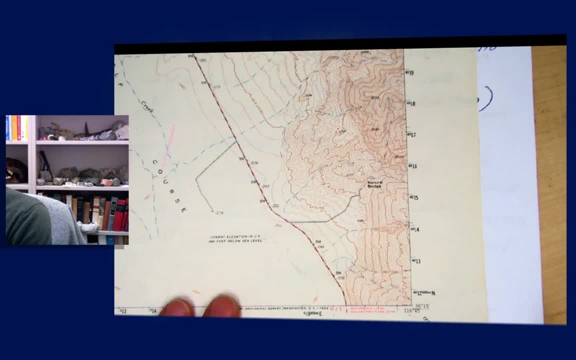 So the southern part of the map is here at 3615, right. So the difference between that is 15 minutes. between 3615 and 30, that's 15 minutes. So usually degrees are these little circles and 15 minutes is one tick mark there, Provincetown Quadrangle in Massachusetts, and you can see it's. 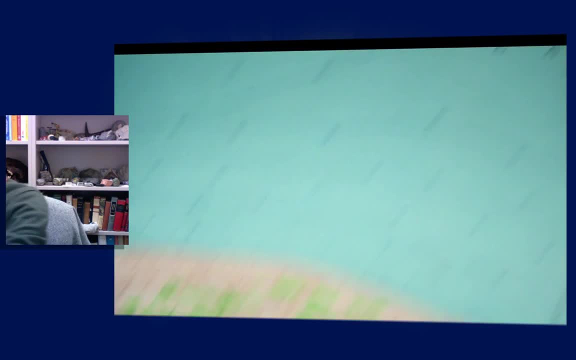 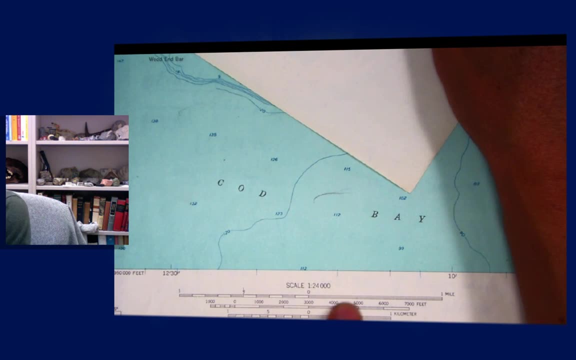 a seven and a half minute series, and so we'll look at that and we'll see what we've got here. So this one for its scale down here it shows right away that it's 1 to 24,000.. You can also see the graphic bar scale right in here. Now what does that mean? We need to be able. 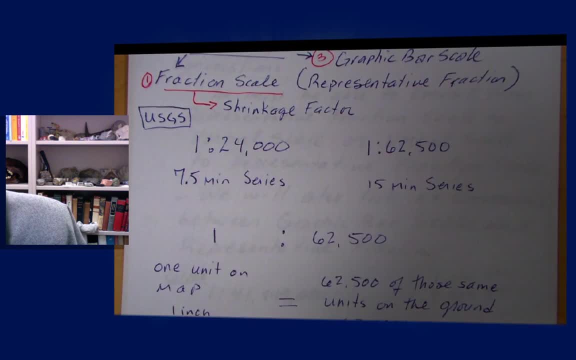 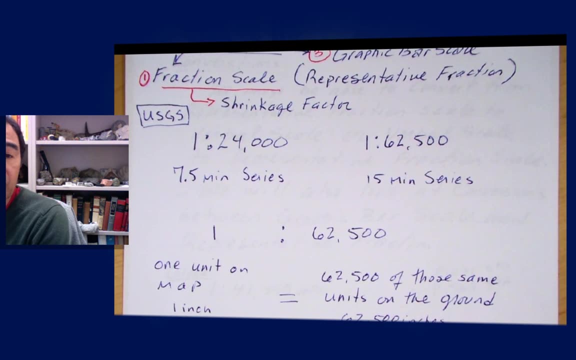 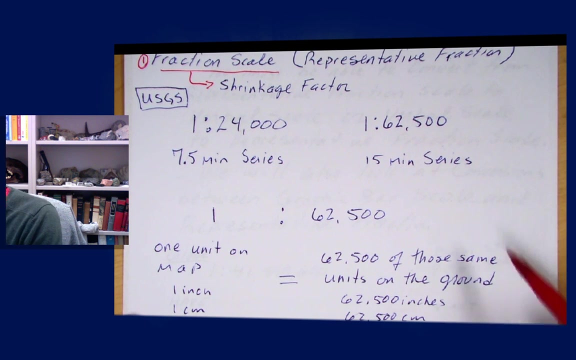 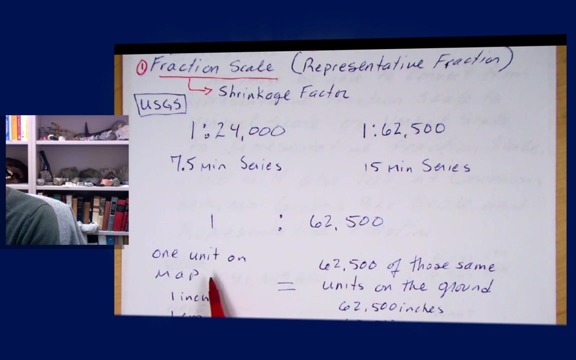 to convert between these graphic bar scales or representative fraction scales to a stated ratio, a verbal scale that will make sense to us. So let's think about this fractional scale or representative fraction first. So what it means? it means that for every one unit measured on the map, one unit measured on the map, it's going to be equivalent to: 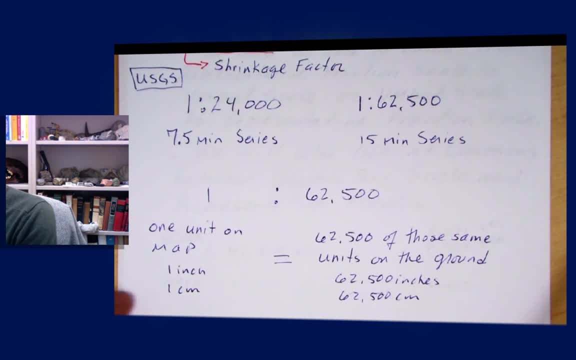 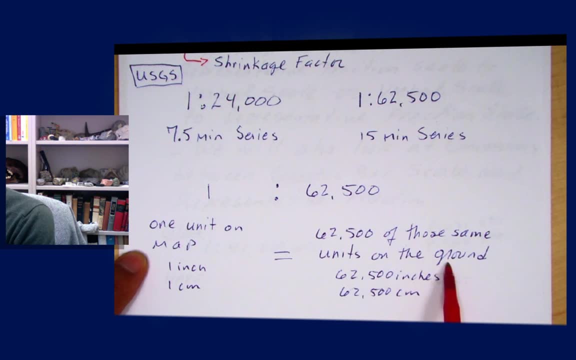 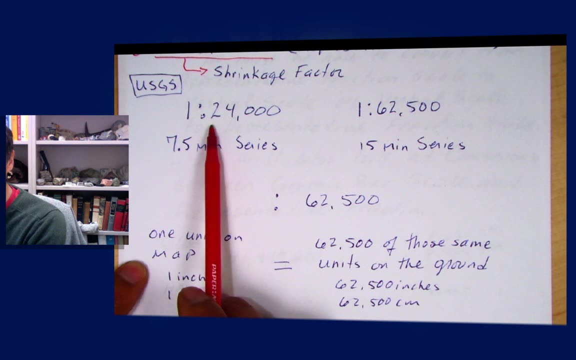 those same number of units measured on the ground. So one unit on map here equals 62,500 of those same units on the ground. So if I'm looking at the seven and a half minute series, if I measure one unit on the map I'm really covering 24,000 of those same units on the 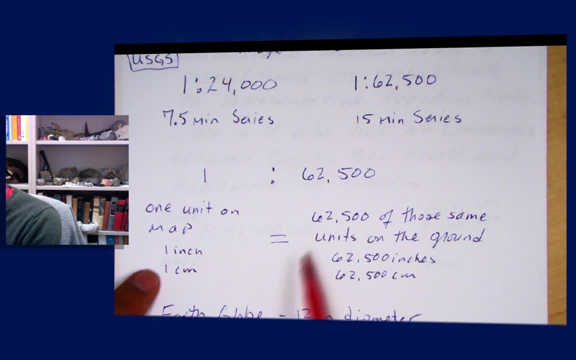 ground. So for example, on this one here for the 15 minute series, one inch on the map covers those many inches on the ground. I can use centimeters because it's a unit-less ratio. So if one centimeter on the map will cover those many centimeters on the ground, 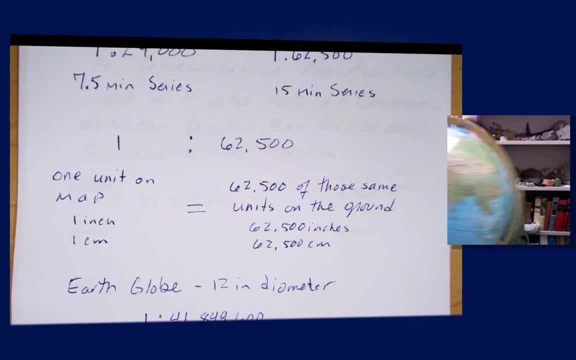 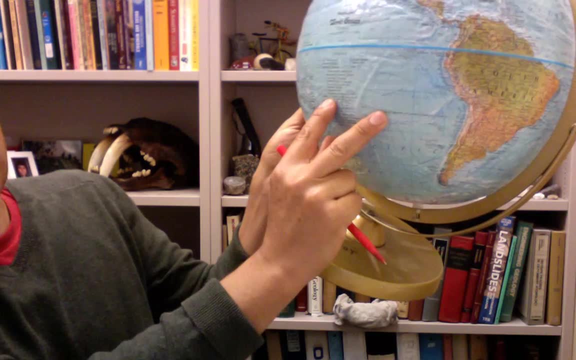 I also have an Earth globe over here. We'll look at the globe, And this globe is a 12-inch diameter series. If you look down here, it does give me a verbal- not a verbal, but a representative- fraction, And so we basically have to shrink down the 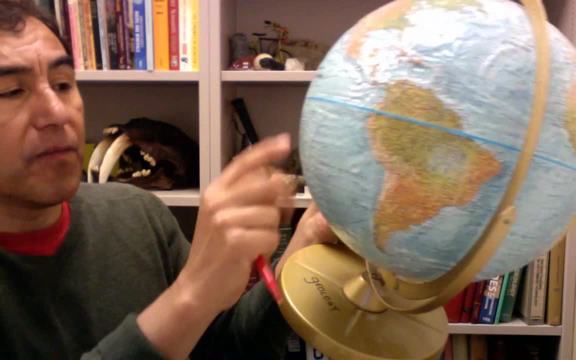 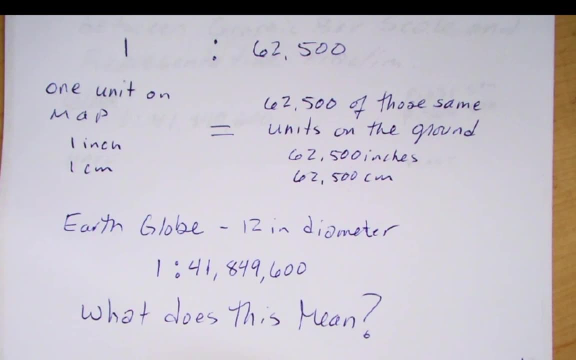 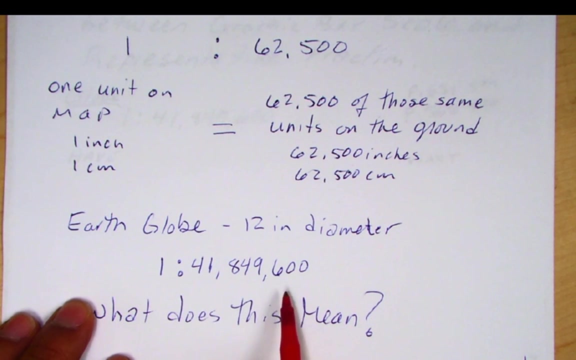 planet to fit on this 12-inch diameter globe, And we shrink it down about 41 million times. So if we look at this scale here- I wrote it down- So it's one ratio to 41,849,600.. So what does that mean? And so we need to convert it into something that makes sense. 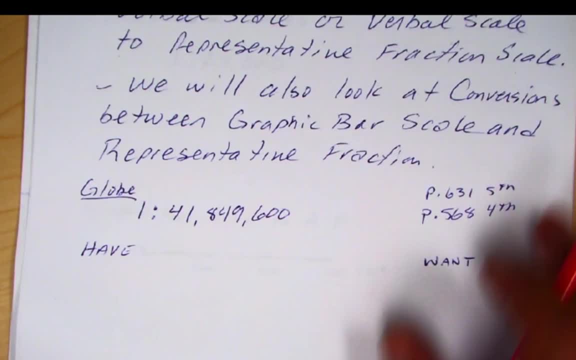 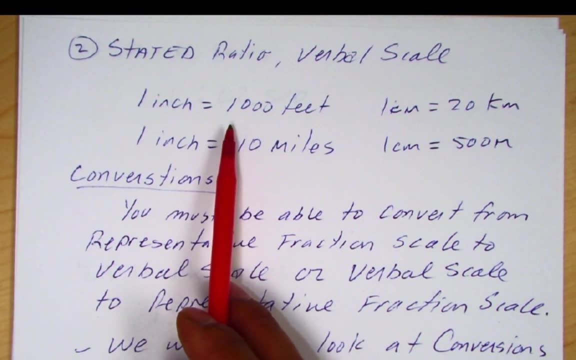 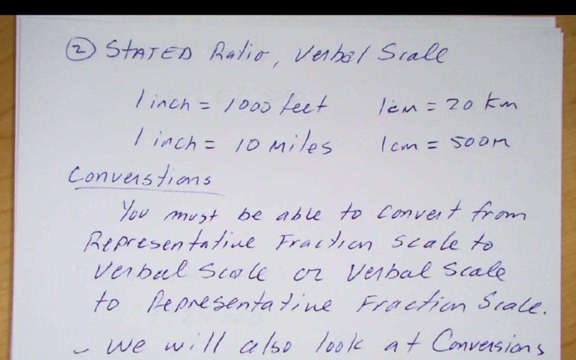 to us. So that's where this stated ratio scale comes in. We wanted to say it's like one inch on the map is 10 miles or one inch is 1,000 feet. That makes sense to us. One centimeter is 500 meters. We can relate to that more easily than one ratio to a bunch of numbers. 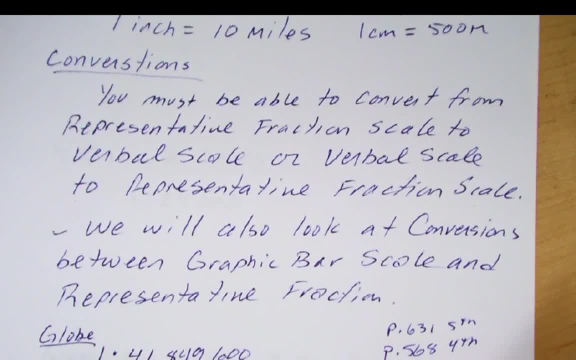 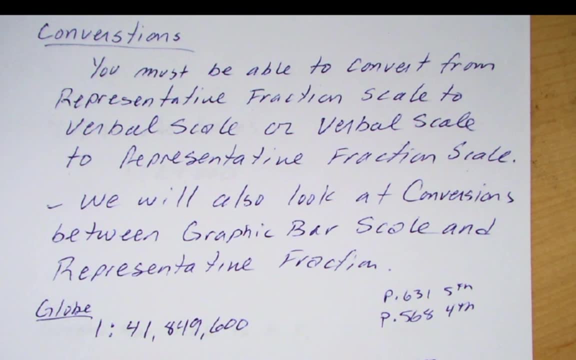 So we need to make these conversions. You must be able to convert from representative fraction scale to a verbal scale or from the verbal scale back to the representative fraction scale, And I think a couple of problems in the lab I noticed deal with converting between the graphic bar scale and representative fraction. So we'll look at some examples of 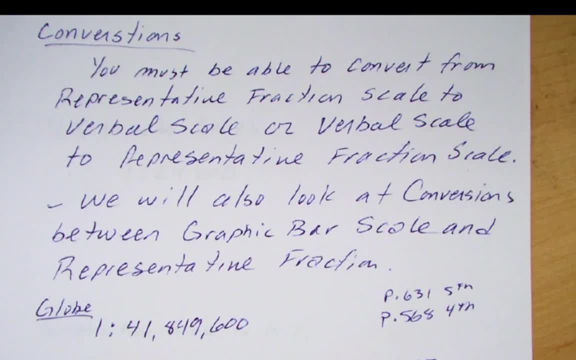 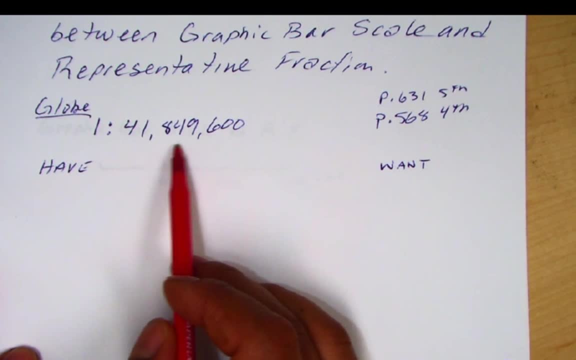 that here in a little bit. So let's go back to our globe. So remember, the globe scale was 140, one ratio to 41,849,600.. So what does that mean? We want to know. we want to say one inch equals 1.. 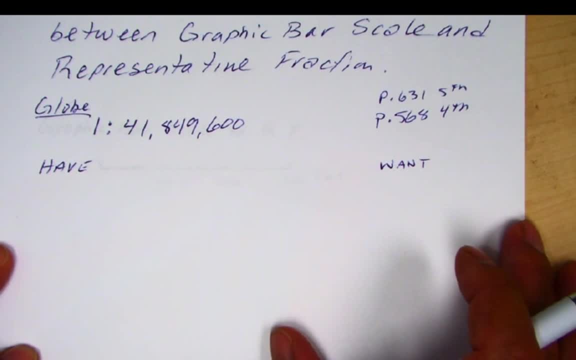 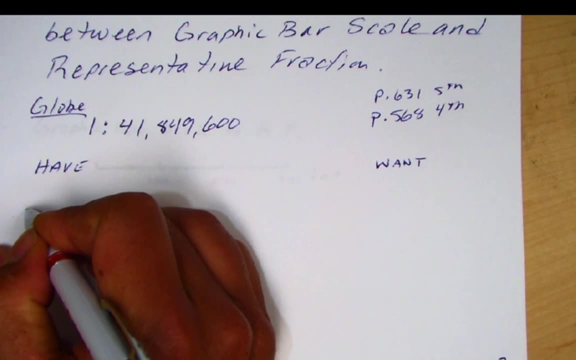 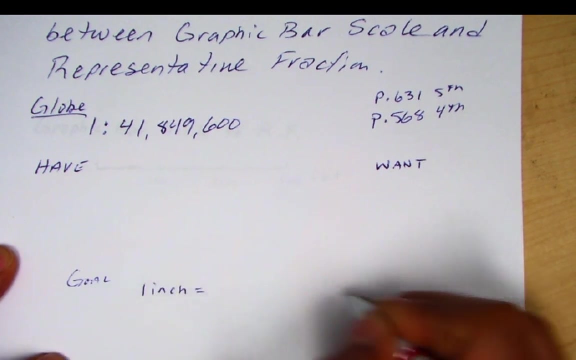 Some number of miles, right? So I always break it out like this whenever I do these conversions: What do I have? Well, I have a whole lot of inches here, right? So remember I'm going to go inches. So my goal here is: one inch equals some number of miles, right? 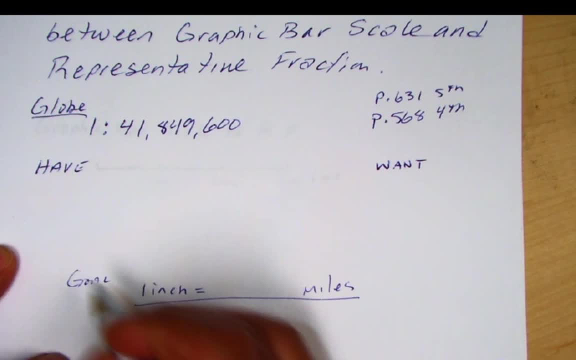 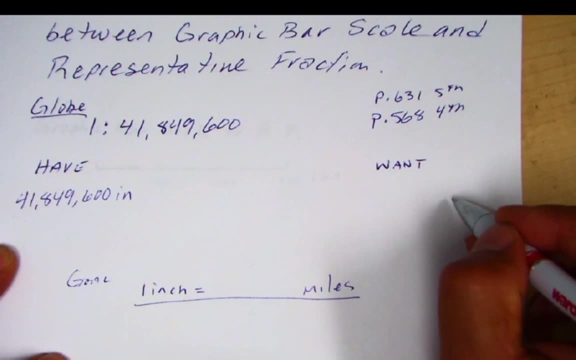 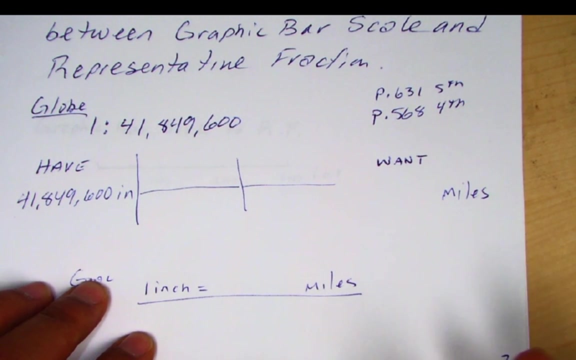 So that's what my goal is. So what I have: I have a whole lot of inches. I have 41 million. I have those many inches Over here. I want miles, And so I'm going to break this out in usually two, maybe three. 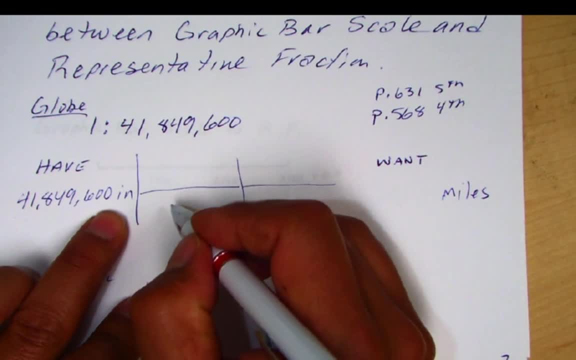 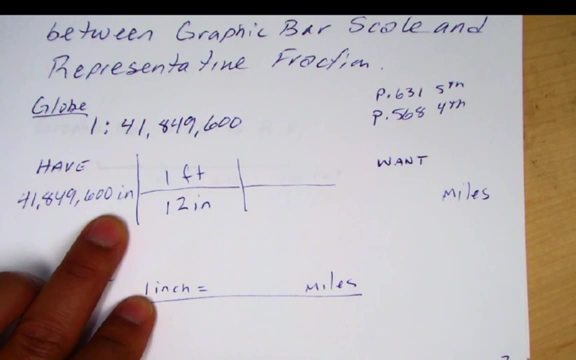 steps. So first of all, I want to get rid of inches. So I know that 12 inches equals one foot, So that's going to allow me to cancel out these inches right. So now my answer is going to be in feet. Then I want to get rid of the feet, So one of the magic numbers. 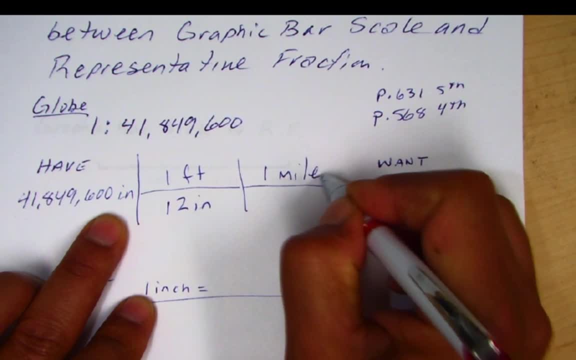 is: I know that in one mile there's five feet. So I want to get rid of the feet, So I want to get rid of the feet. So one of the magic numbers is: I know that in one mile there's 5,280 feet. That's something you're just going to have to memorize or write it down. 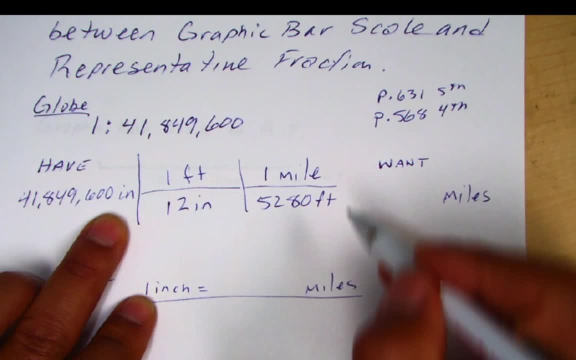 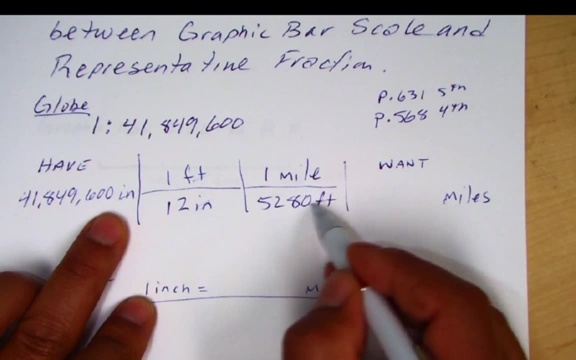 somewhere. One mile is 5,280 feet, right? So what's going to happen? I'm going to cancel my feet out here and my answer is going to be in miles, because inches go away, feet go away and my answer will be in miles. So if we do the calculations here, so we'll take. 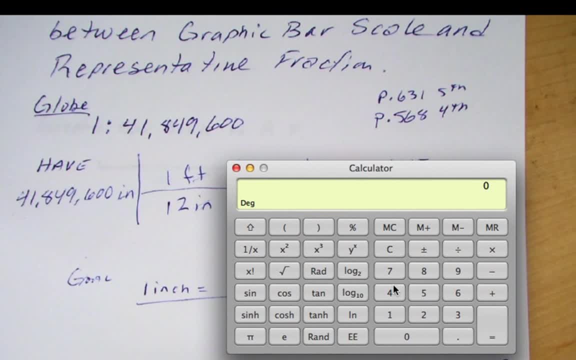 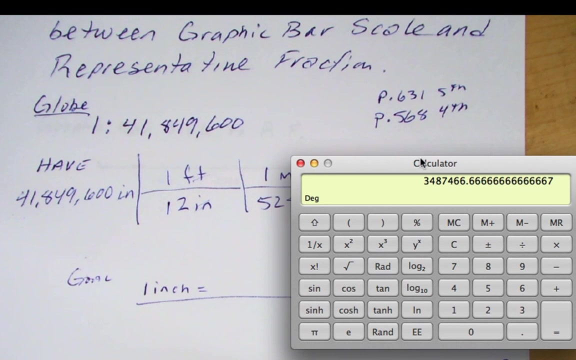 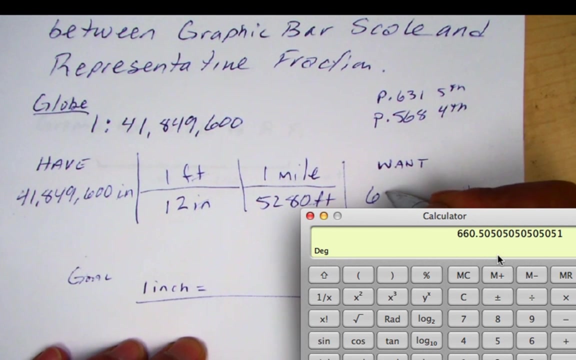 the 41 million 41,849.. 600.. And now it looks like we have to divide. We have to divide by 12, right? And then we have to divide that number by 5,280, 660.5.. So we'll just round it to 660.. So it's 660.5.. 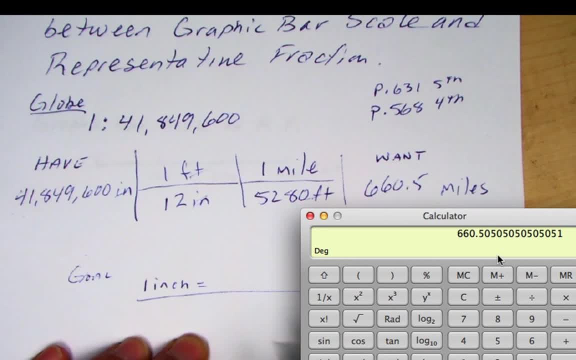 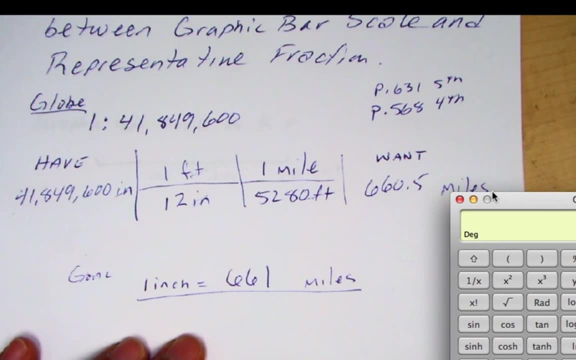 In fact we'll round it to 661.. And so in this case it's 661 miles. So that's how much we can do. So now, that makes sense to us. So this would be the verbal scale. So we've just determined. 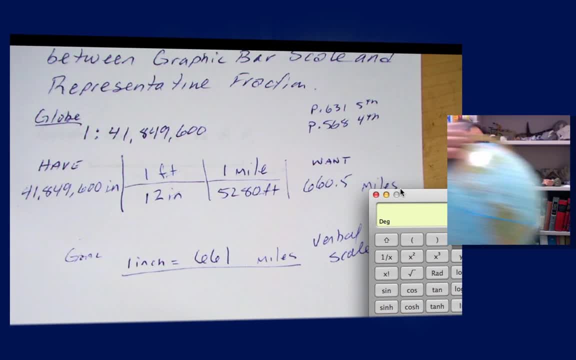 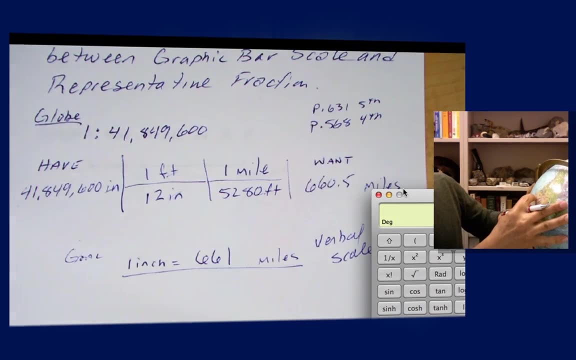 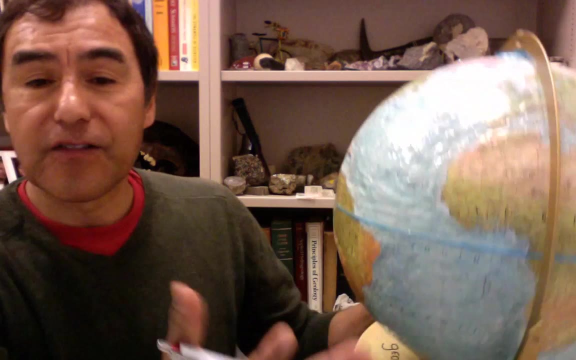 that on this globe, one inch is about 661 miles, And if you think about one inch, that's about the distance from San Francisco to Tijuana or so that's about 600 miles. Yeah, so that makes about sense. So that's how we can go from representative to fraction to this verbal. 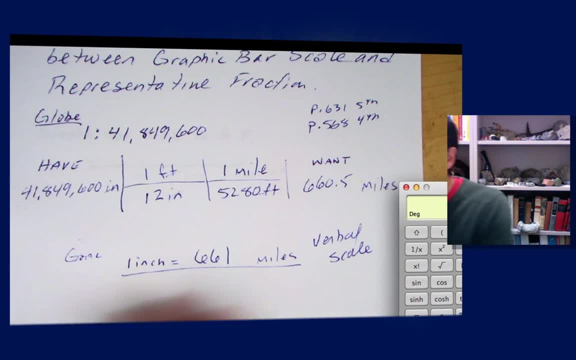 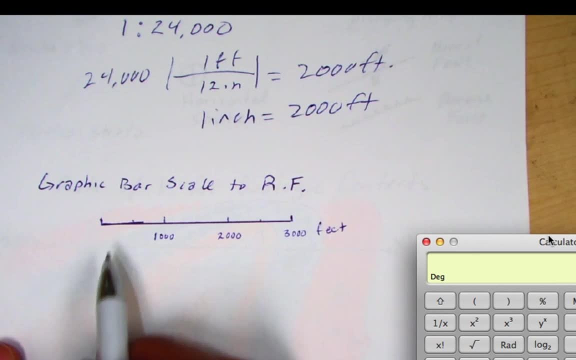 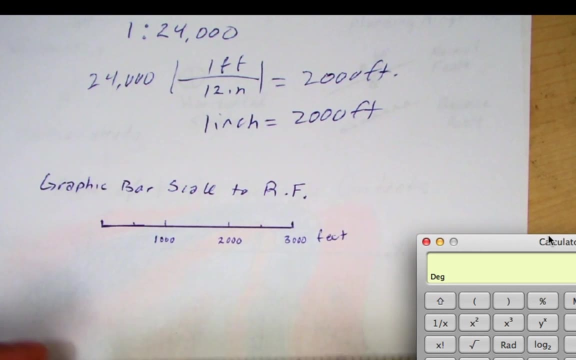 or stated ratio. Now let's keep looking here. We want to convert between a graphic bar scale- you have a bar scale- and the representative to fraction. So I see right away here that one inch, so I can get my ruler here, and I can see that one inch here is 1,000 feet, There's one inch. 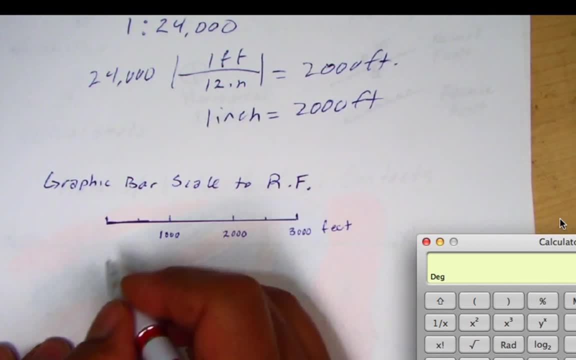 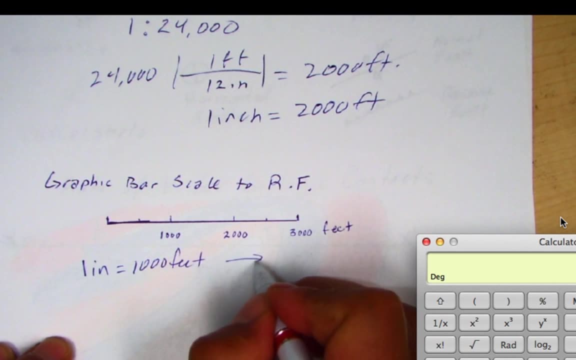 is 1,000 feet, So I'll write that down. So, based on the graphic bar scale, one inch is 1,000 feet, So I want to convert that to that representative fraction. So this is going to take me backwards. 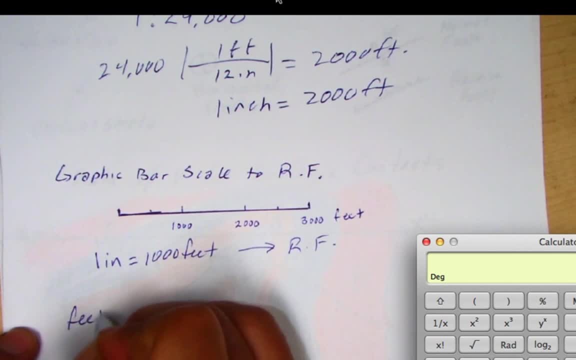 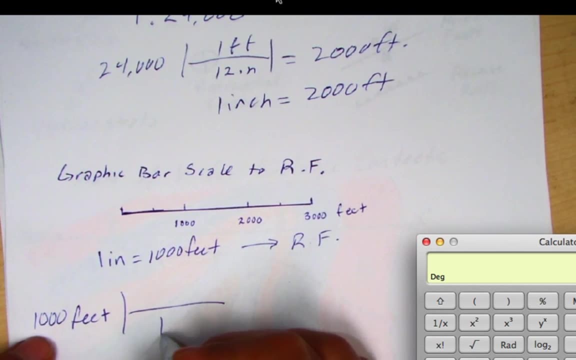 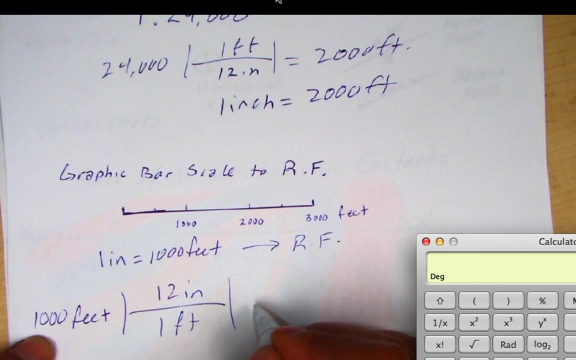 So here I have feet right. In fact I have 1,000 feet, And so I know that in one foot there are 12 inches right One foot, there are 12 inches. And so to do that, I'm going. 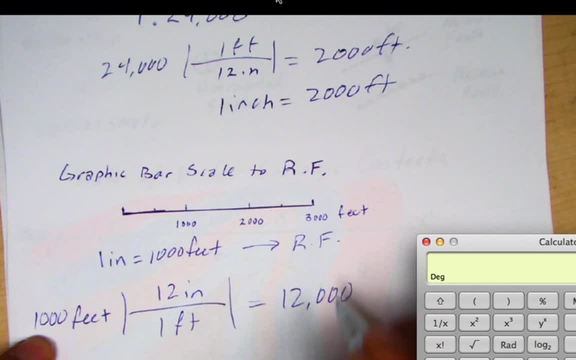 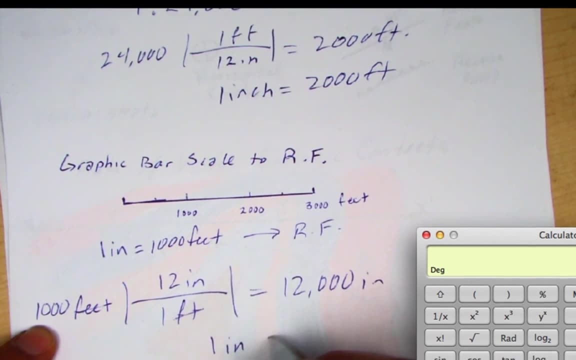 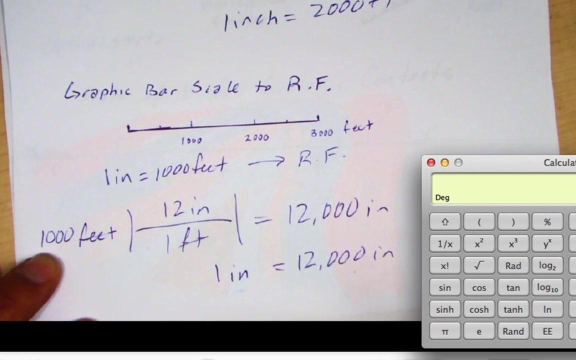 to: basically this is going to be 12,000, right, I just multiply these across Feet, cancel out. So this is going to be inches. So now I have, one inch equals 12,000 inches. So one inch on the map is 12,000 inches on the ground. Well, that's my representative to fraction. 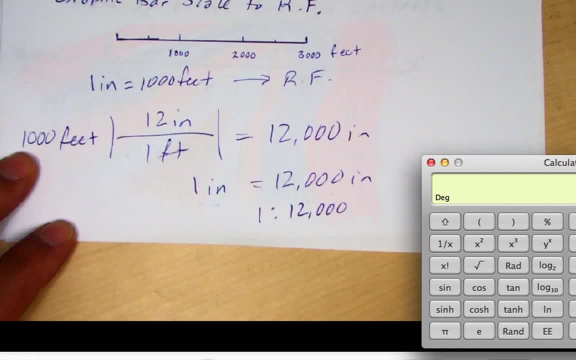 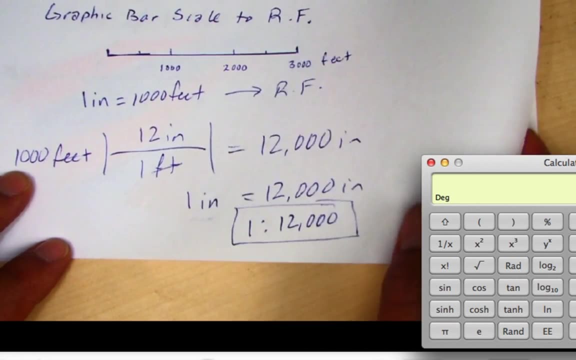 1 to 12,000, right, So that would be the final answer. right there, the representative to fraction. Let's do another example. Let's say we measured a different one, just to kind of show We'll go for miles here. 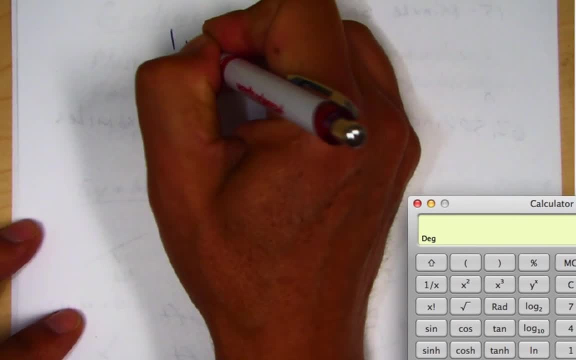 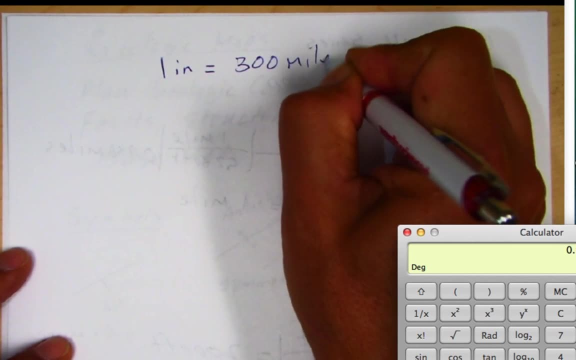 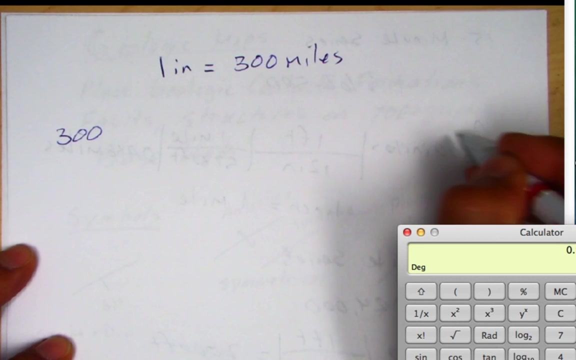 Let's say our map had one inch equals. let's say it's 300 miles. So that's a verbal stated ratio, right? So now we'll have our 300 miles. Remember, we want to go to inches. We want to make this into inches over here. 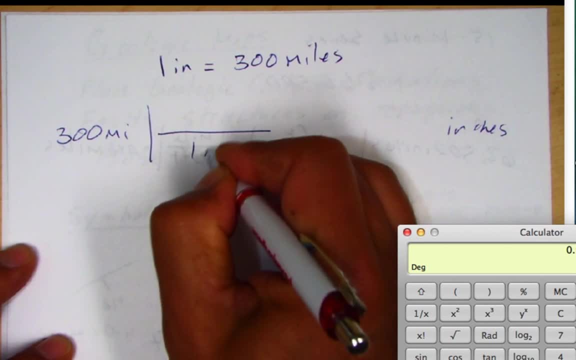 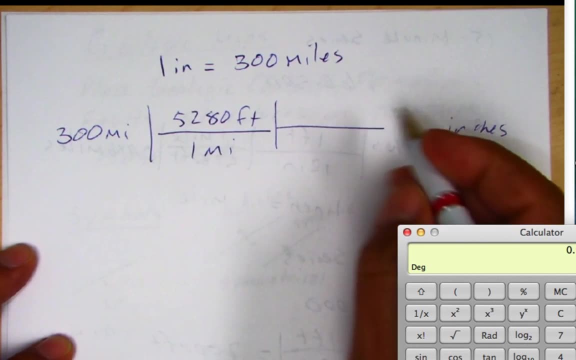 So the first thing we want to do we want to get rid of those miles. So in one mile there are those 52,800 feet, And so that'll get rid of my miles here, And I know that in one foot there are those. 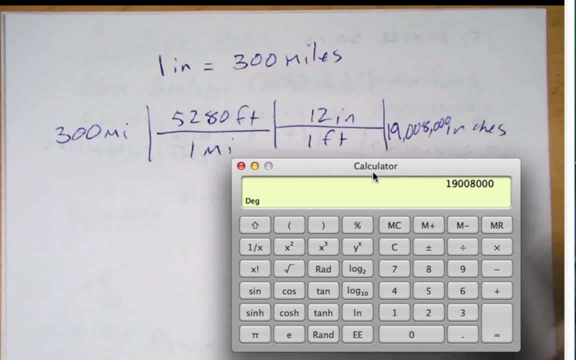 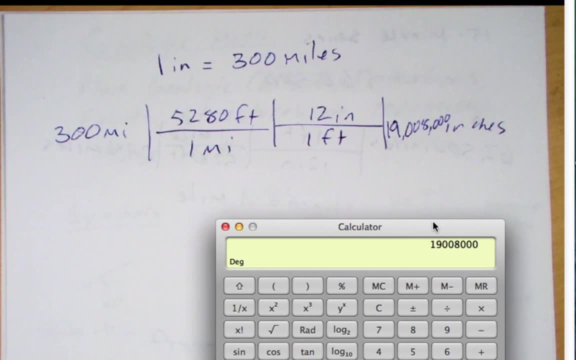 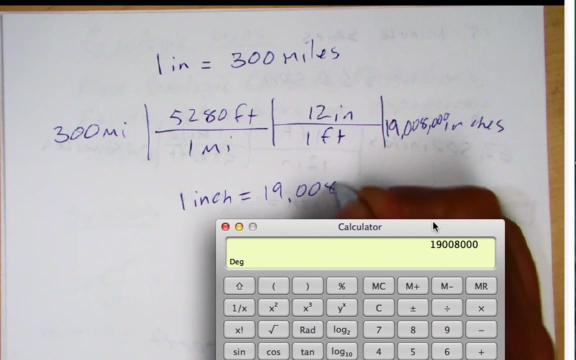 12 inches, right? So it's basically the same idea, but going backwards. So this basically turns out to 19,008,000 inches. 19,008,000 inches, And so that means one inch equals those 19,008,000 inches, right? So our representative to fraction would be: 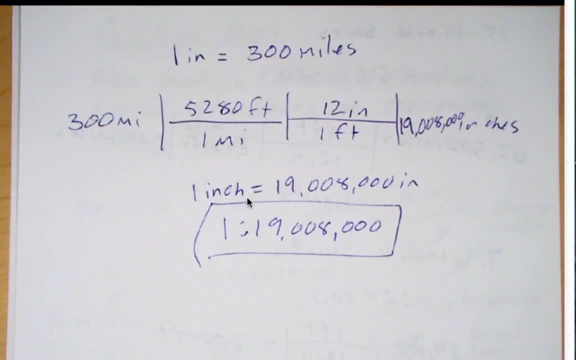 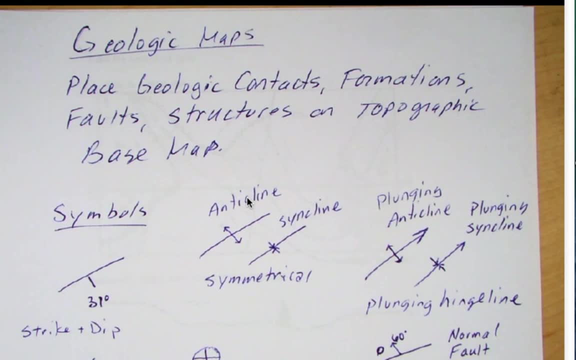 one ratio to those 19. So you should be able to make those conversions. Now let's look at geologic maps. And so geologic maps are where we want to place geologic contacts, formations, faults, structures on a topographic basement. 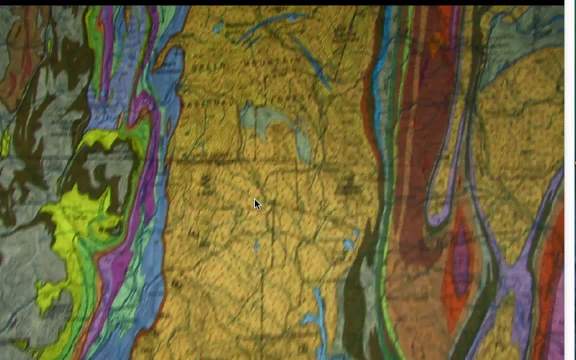 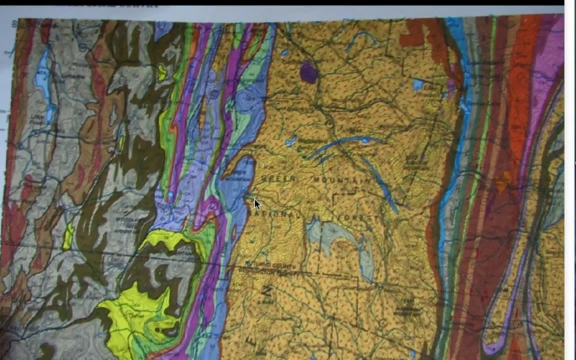 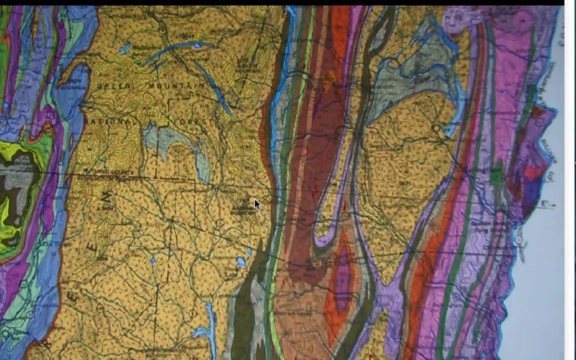 And here I have a geologic map of Vermont right. So here's from the Vermont Geological Survey And you can see there's all these colors, And the colors represent different geologic formations. There's symbols, And usually each geologic map will have a key, And so 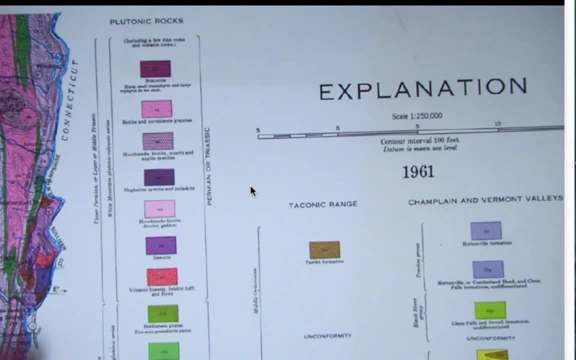 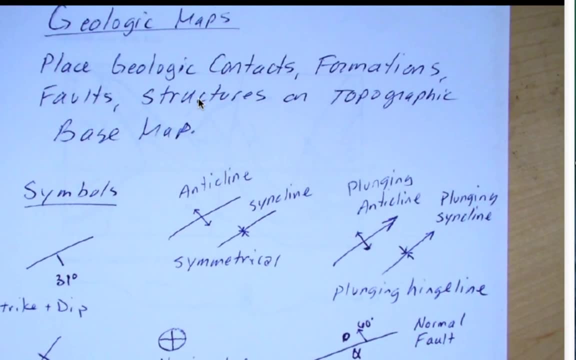 you can see, there's a key here: an explanation showing the different rock units, their ages. To do this, to make maps, we need to use geologic symbols, And these are going to be a little bit different than the topographic maps, And so I've already explained a little bit about. 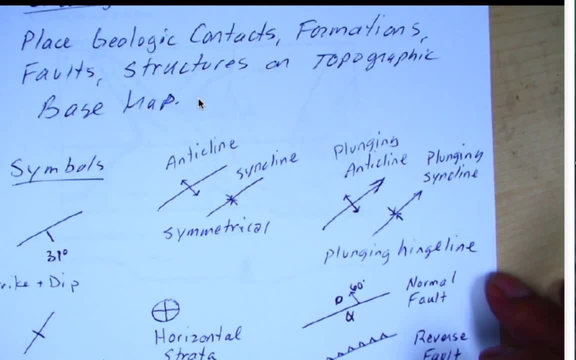 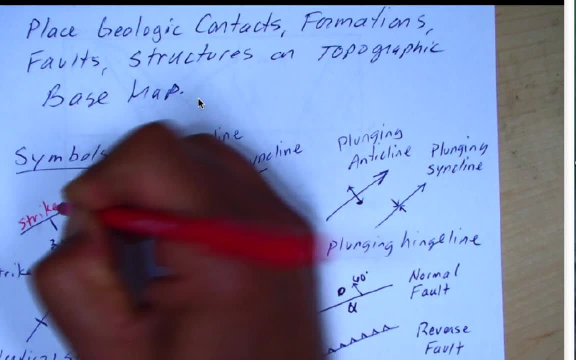 strike and dip. So that's one of the really important ones here. So remember, the key thing is that this line right here is the strike line, That line is the strike line And then this little tick mark is a dip. So remember, dip is always. 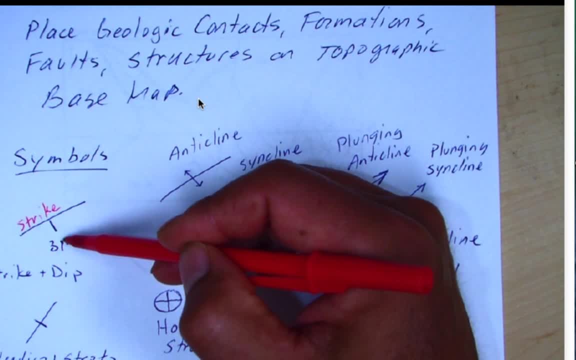 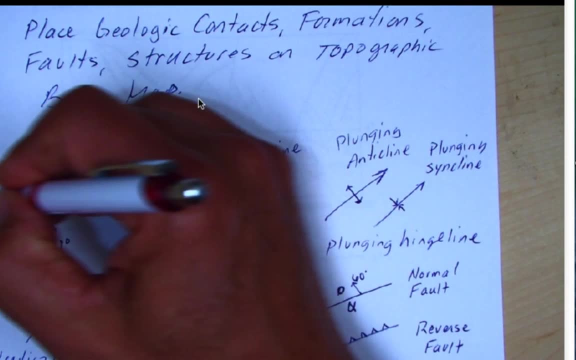 perpendicular to strike. And here it's telling me it's dipping down here to the southeast at around 31 degrees. So remember, if we had a compass rose, let's say north, usually most maps will have north going straight up, So there would be a north line going straight. 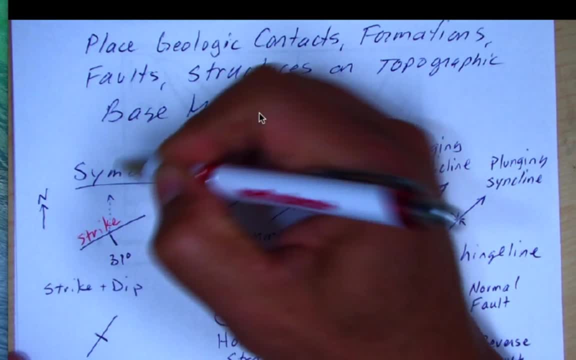 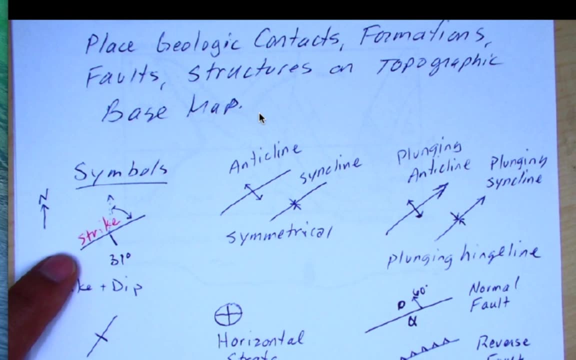 up right here. That would be the north, right there. So my goal is to measure this angle to figure out the strike, Because remember the way this strike line is drawn: it's drawn according to its orientation, So we never put the numbers here, We just draw the line. 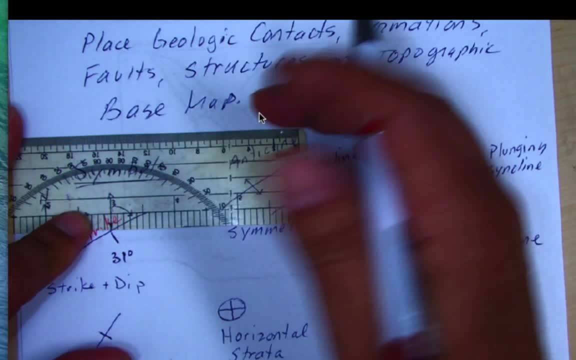 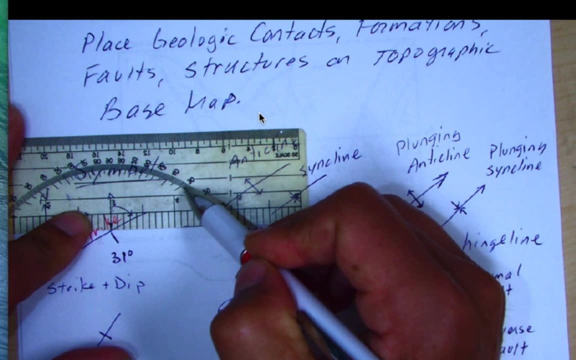 So on this one here, if I measure that angle, I put my bullseye right at the corner. I'm going to measure this angle here. I see it goes 10, 20, 30,, 40,, 50, 60.. So going out here to about 60. 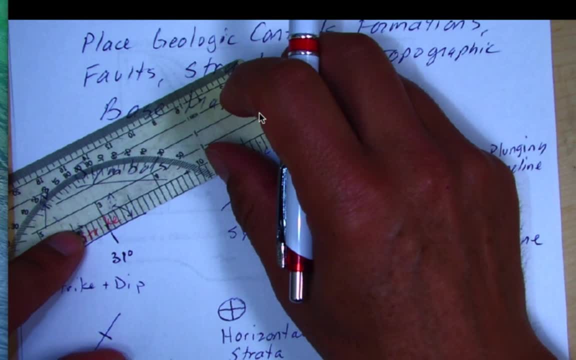 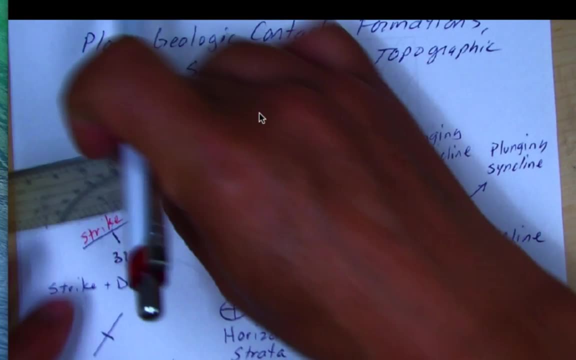 So another way I can do it, I can place this horizontally here and then follow this strike line straight up, and it goes up to 60.. I kind of have it backwards there, but let's do it this way, So I can put it right there and I see that it goes 10,, 20,, 30,, 40,, 50, and this north. 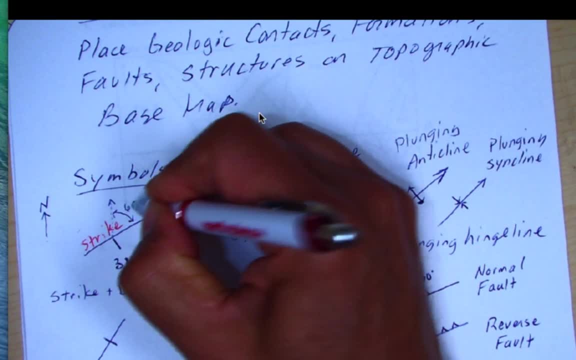 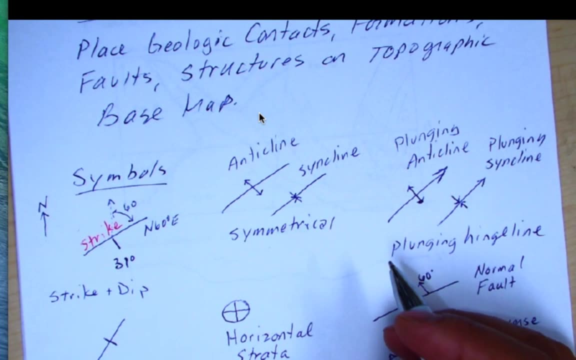 goes right to 60. So this angle is 60 degrees. So the strike of that line is north, 60 degrees east, because I went toward the east direction. So that's how we do strike, But strike will always be drawn on. 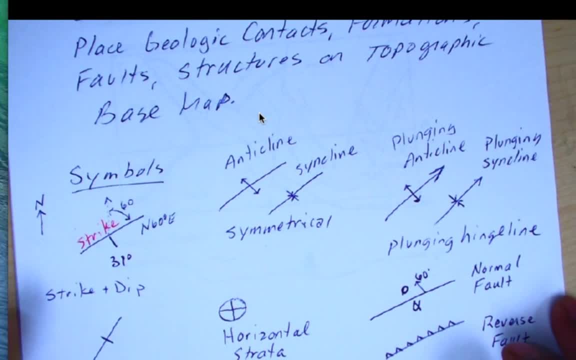 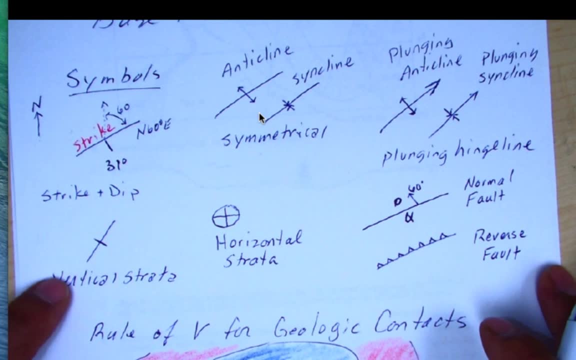 the geologic map. according to this, You never really draw this, You just draw that line. And then other symbols that we use to strike and dip are for vertical strata. That means these are: this symbol here means that it's dipping 90 degrees, It's vertical. And then 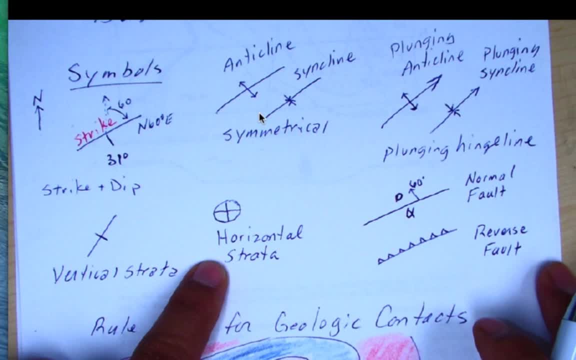 over here: horizontal strata. we show this bullseye. So that's like if you go to the Grand Canyon, pretty much everything's horizontal: The Kaibab, Coconino sandstones, those are. they're going to have horizontal strata here. 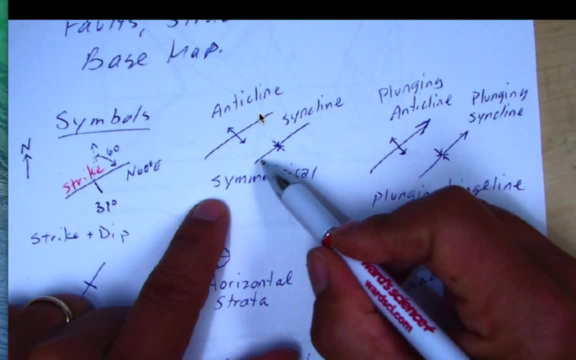 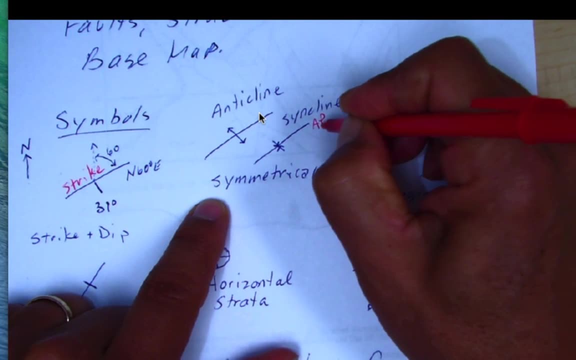 I talked about anticlines and synclines. So if they're symmetrical we'll have just the axial plane. So remember this line: here is the axial plane, And then here they're dipping toward the axial plane. so that's a syncline. Dipping away, that's an anticline. 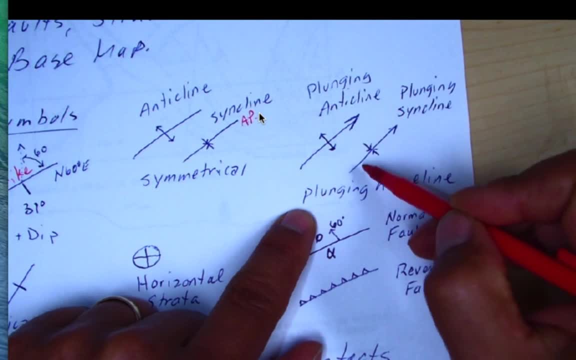 Now, if we have a plunging hinged line, you can see the hinged line is plunging here. So we have a plunging syncline here and a plunging anticline there. So we'll actually use these symbols a little bit here. 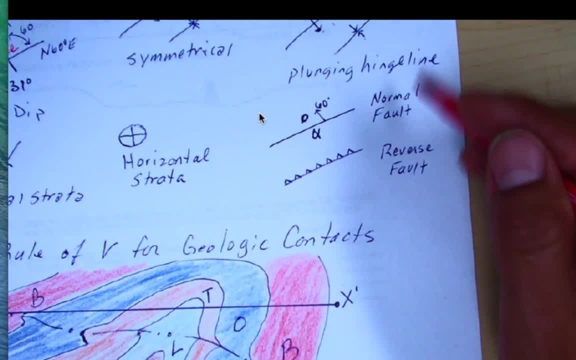 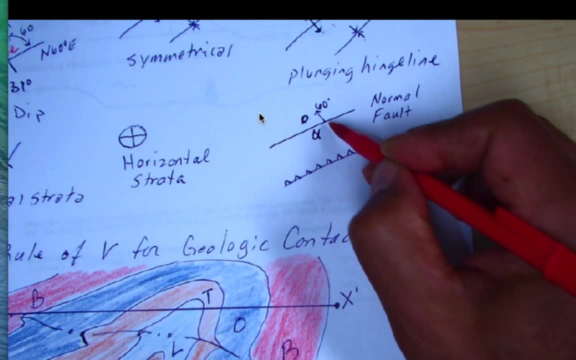 Other symbols. here we have a normal fault. This is going down here, This is going up over here. So down and up, And you can see it's dipping off this way. So this would be the hanging wall and this would be the foot wall over here. So the hanging wall is moving. 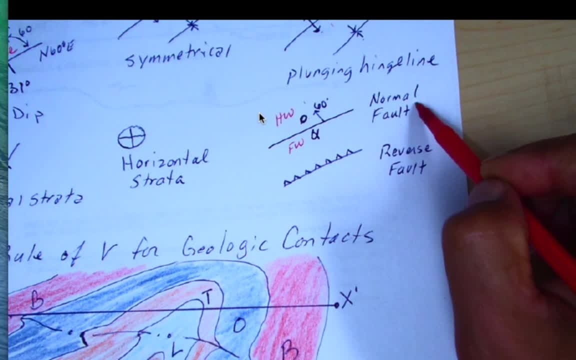 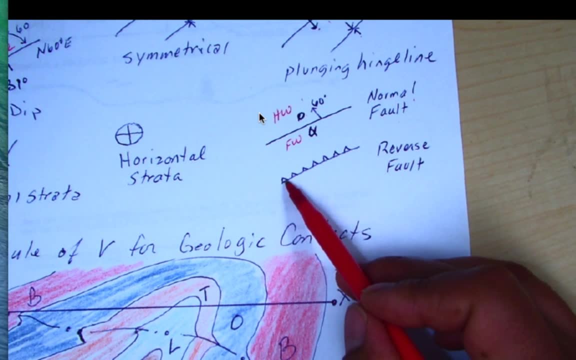 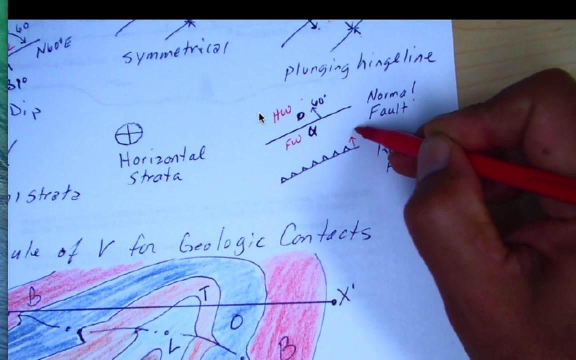 down relative to the foot wall. So that's our normal fault And it's showing us it's dipping at about 60 degrees here- Reverse faults- we show this kind of these teeth on the fault And the teeth always point in the dip direction. So it's dipping down that way. So it's dipping. 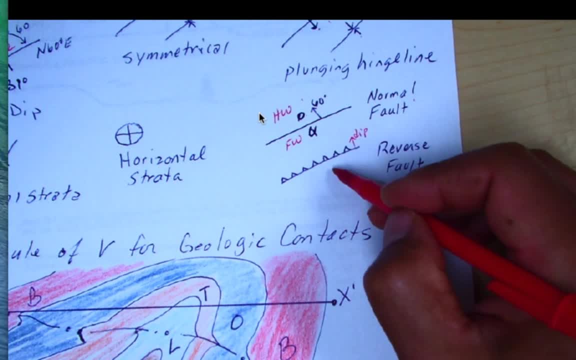 in that direction, And so that means that this must be the foot wall and this must be the hanging wall, And always, where you see the teeth, that's where it's going up and this is going down. So here the hanging wall moves up relative to the foot wall. Well, that's. 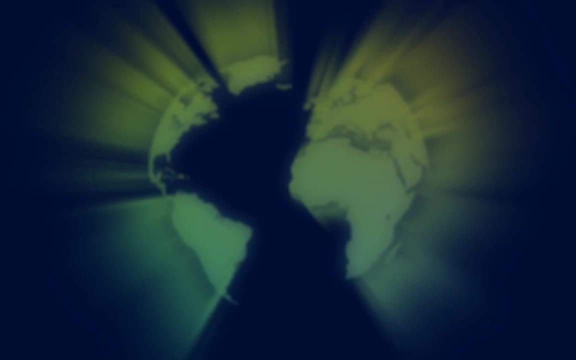 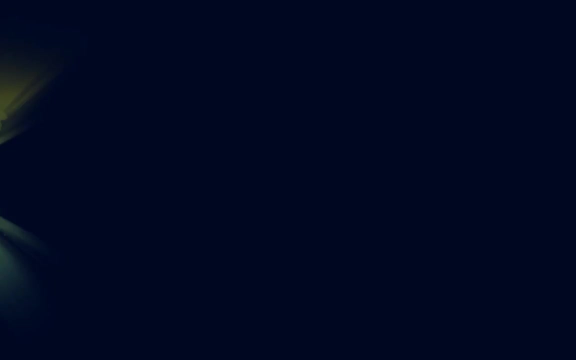 our reverse fault. Reverse fault. Subtitles by the Amaraorg community.